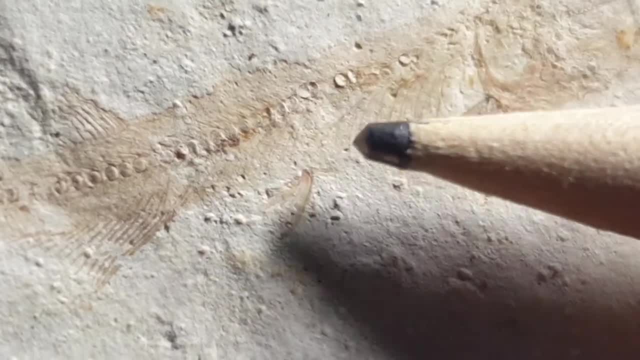 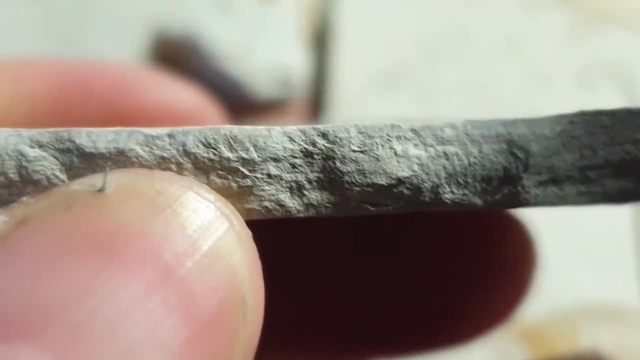 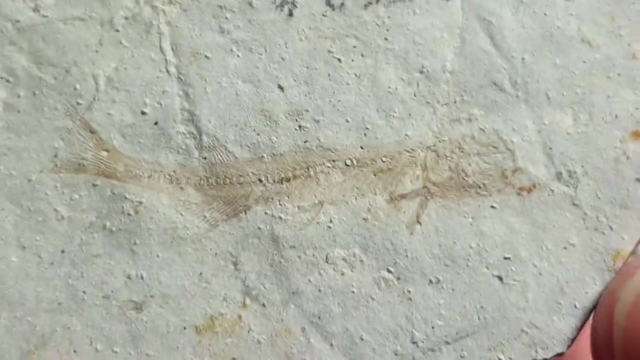 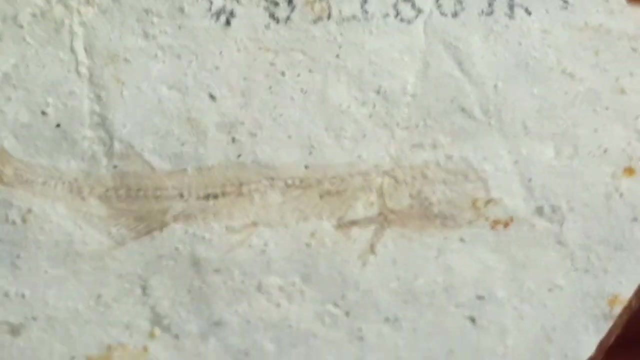 a lot of them have been displaced so they've been pushed on to this side and that's because of pressure. so the pressure of the matrix is this way, so you've got top pressure and bottom pressure. so I'm not too sure if this was layered that way or if this is the upside down piece. it could be either one. 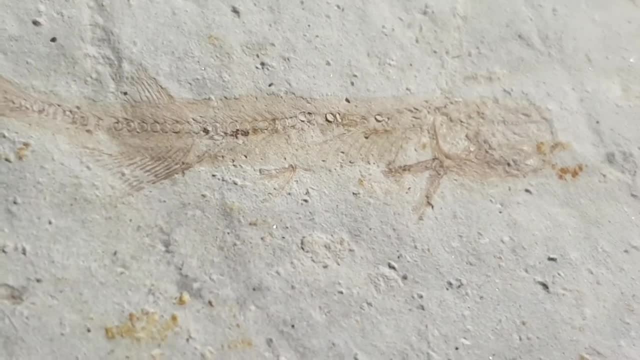 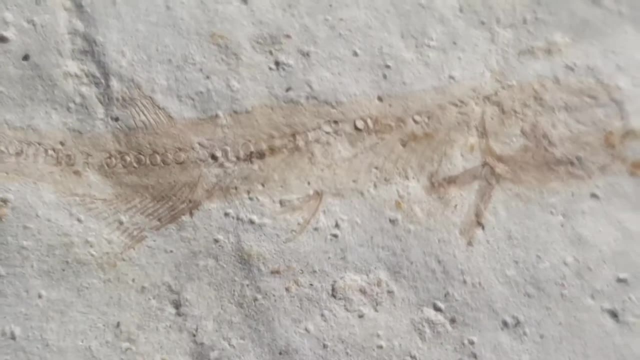 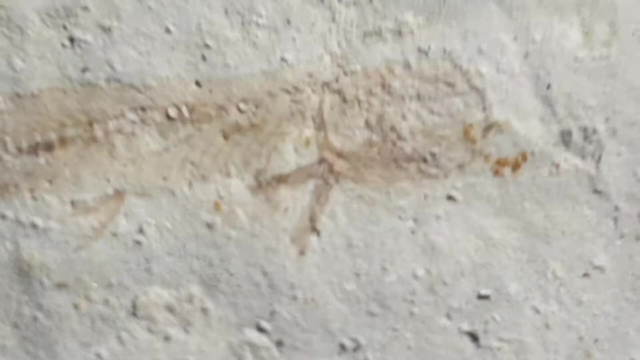 but it doesn't matter, the pressure will be a bit different. the pressure will be a bit different. the pressure will be a bit different usually depending on how much sediment was placed on top. so these are from the lower Cretaceous, so 125 to 135 million years ago, and they're very common. so 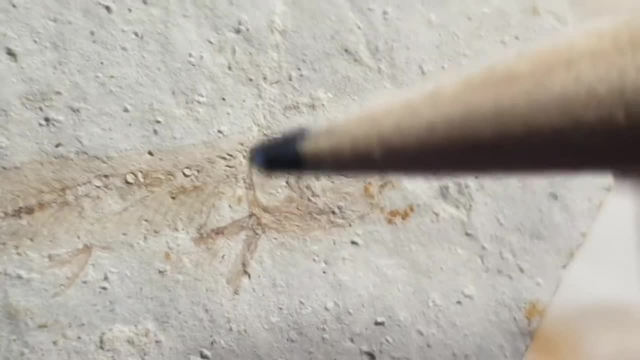 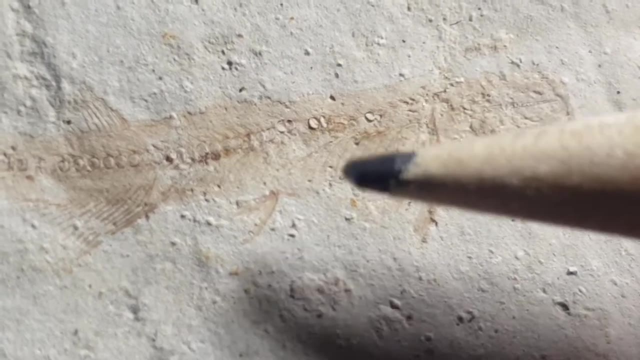 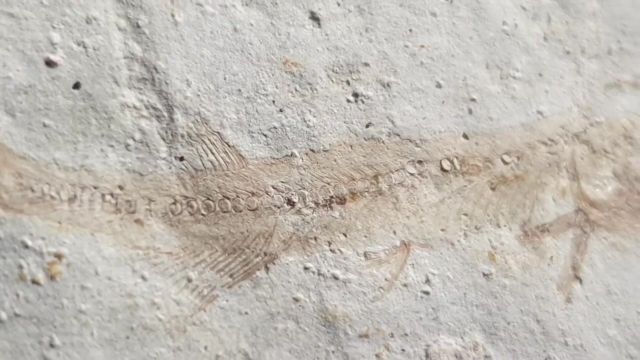 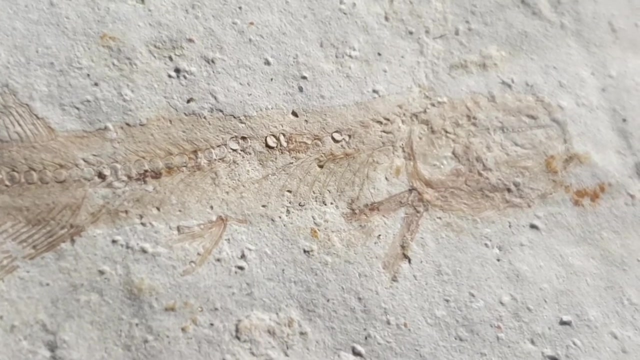 here we have the head, but the head is not really that distinct in this specimen, but the vertebrae is. and then you've got the ribs. so you've got the ribs going along there, a lot of ribcage, and sometimes you can see the internal organs. so this one I can't. and also on 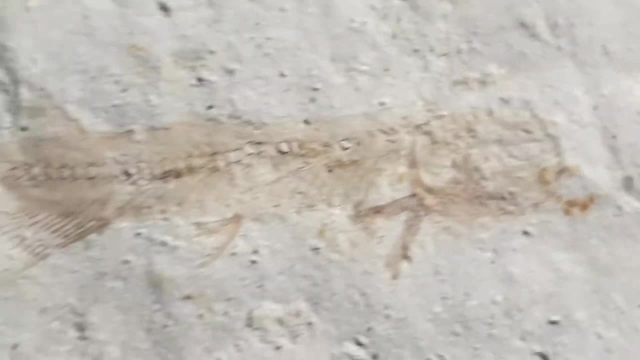 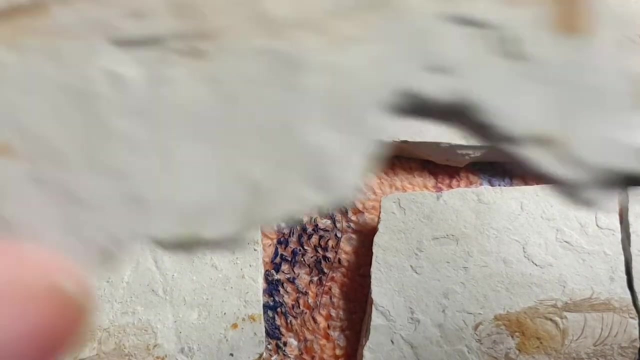 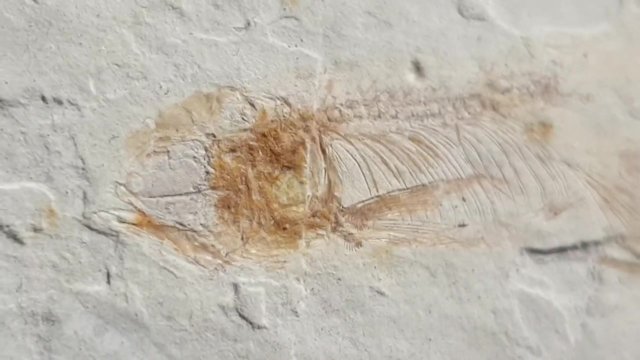 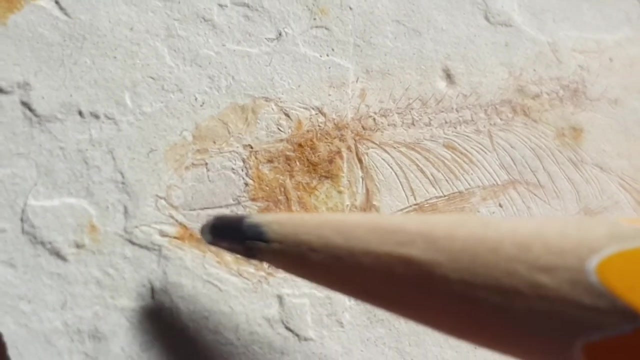 good specimens. you can see the scales. so that will probably be on the other side of this specimen when it was found. but they probably sell them separate. so here we have a head, here we have the eye socket. looks like the eye socket was big, the mandible was there, so we had the 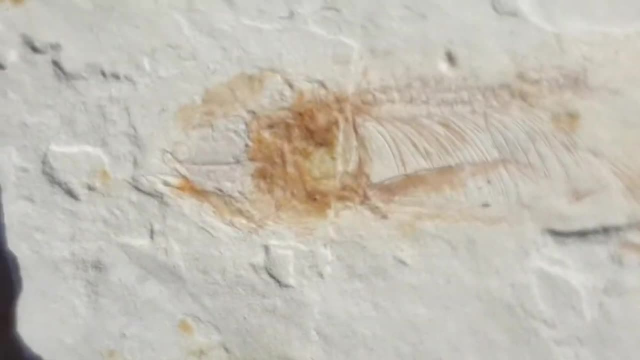 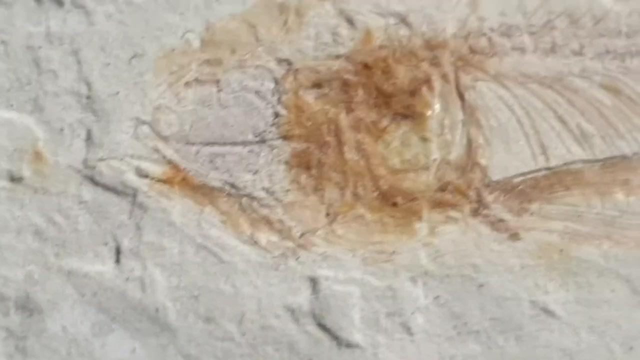 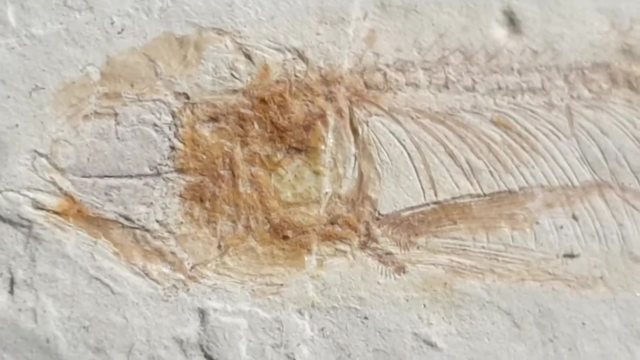 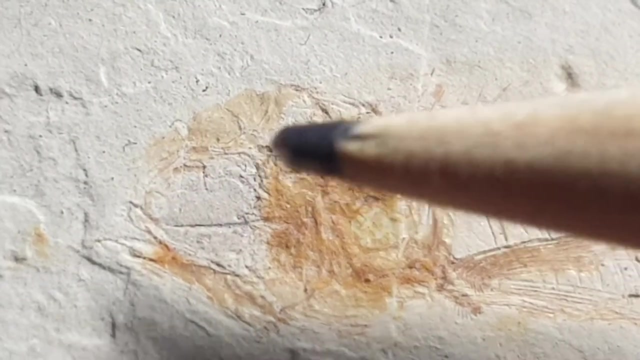 dentary it looks pretty small. so if we just zoom in, yeah, it's pretty hard to see the mandible, the dentary, shall I say. then we have the gill placement is around around here. so this skull, While basics anatomy you can see, You can't really see that much in the anatomy. 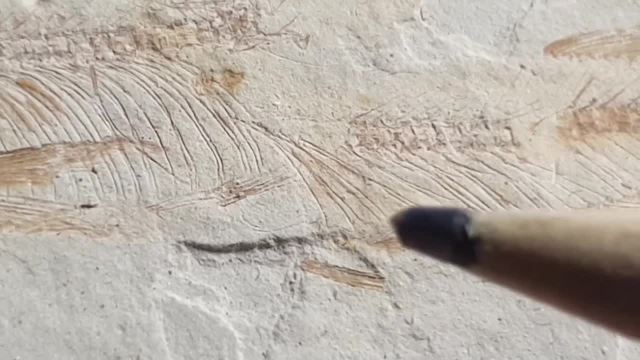 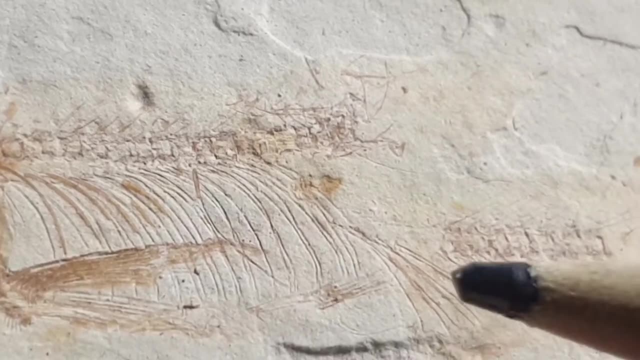 But the ribs, So you can see the vertebrae. This fish has been snapped in half, So the vertebrae stops there And it restarts there, So this has been displaced. Then you've got the ribs, Then you've got the fins as well. 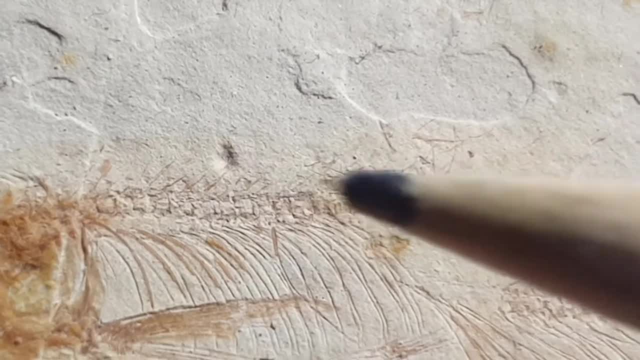 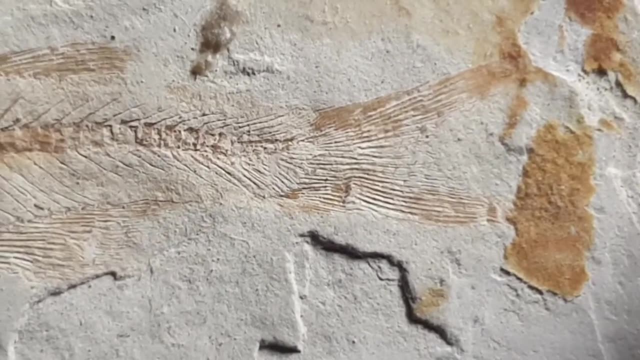 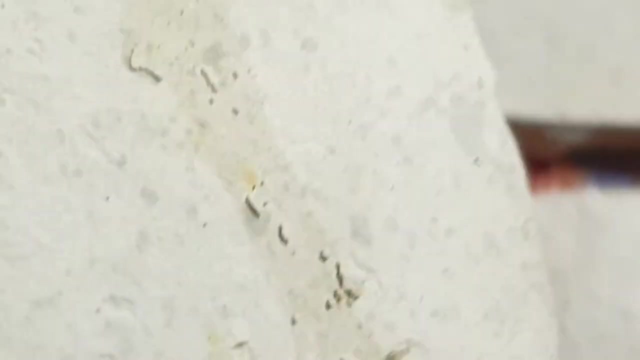 And I don't see a first dorsal fin, I just see the last dorsal fin, So that is a lot better detail. And this one was broken in half. On the bottom we don't find any fossils, So I've got the other piece here. 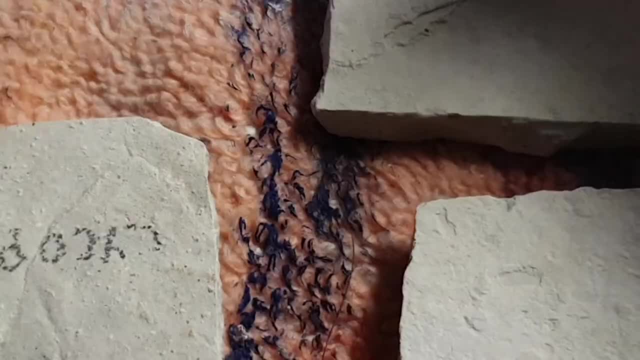 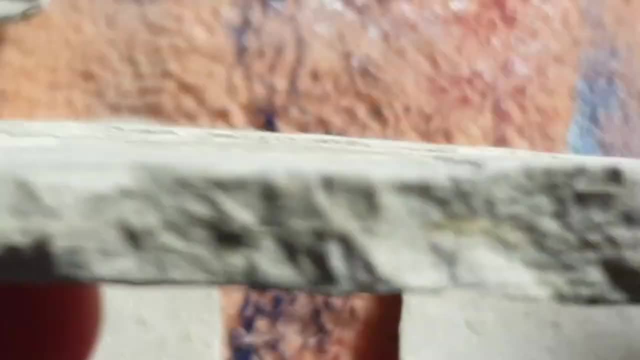 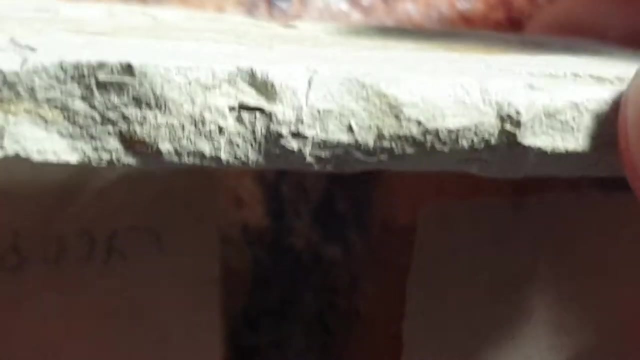 So that's good. If you've got these and they're quite thick, Then you can break them in half And see if there's another fossil underneath, Or if you wanted to look for a fossil, You can. You need to look for dark matrix. 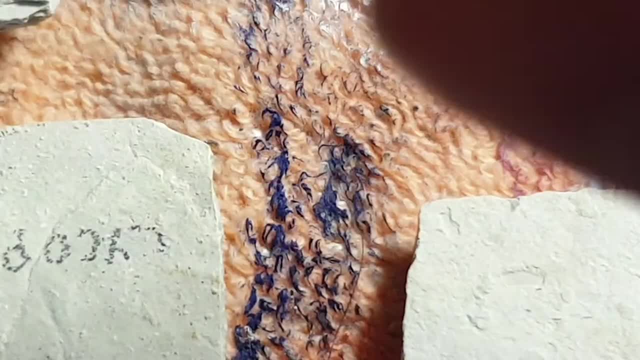 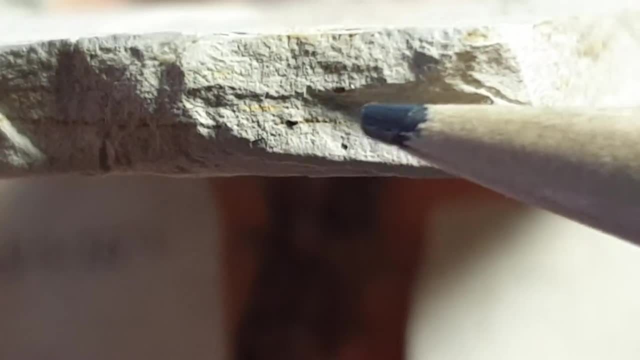 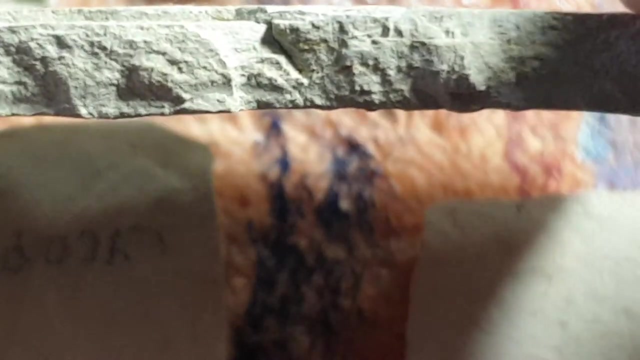 Because you've got laminations in between, So I don't see any dark matrix there. Maybe there could be a fossil in this part here That's been broken in half, But that's how you look for fossils in this matrix: See if there's actually any dark stains. 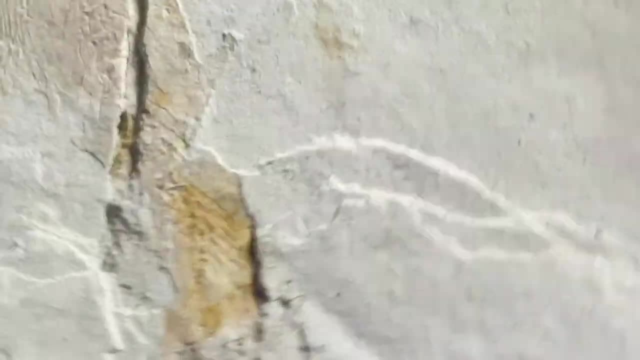 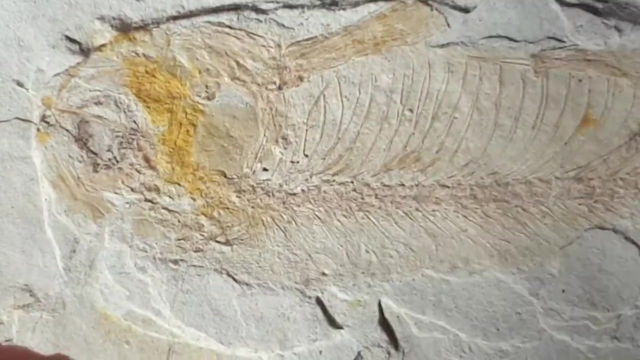 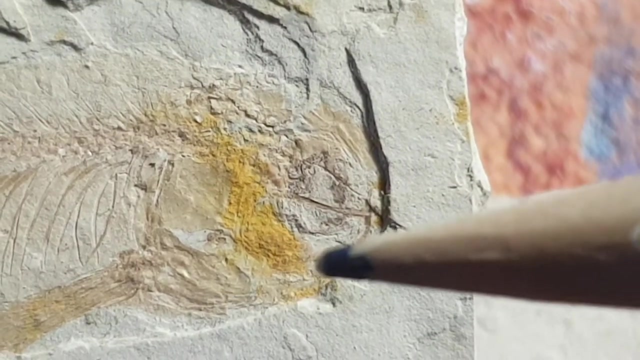 Could be a fossil, Could not be. So this one is a larger specimen, So you can see the eye quite clearly here. It is, if you want it, the upright position. So you've got the eye. The amanda will be somewhere around there. 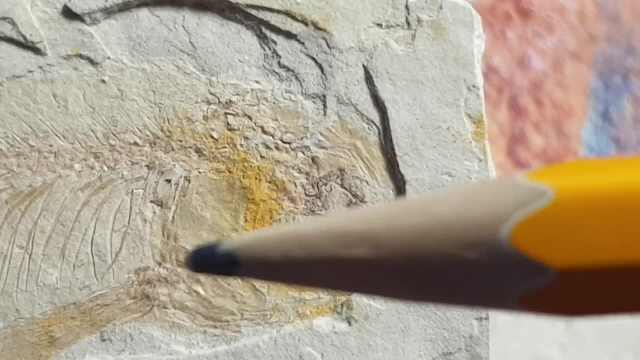 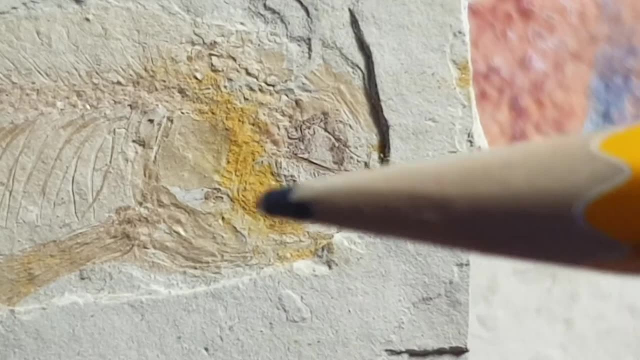 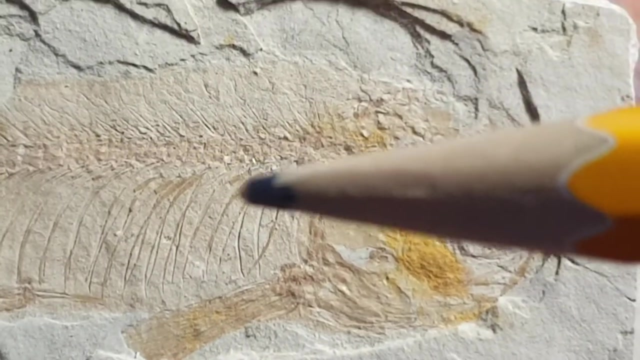 And here we have apple bones. So that's probably the operacle Into operacle as well, But it's hard To see a lot of detail. And the vertebrae starts up here. Then you have the pleural ribs Around here. 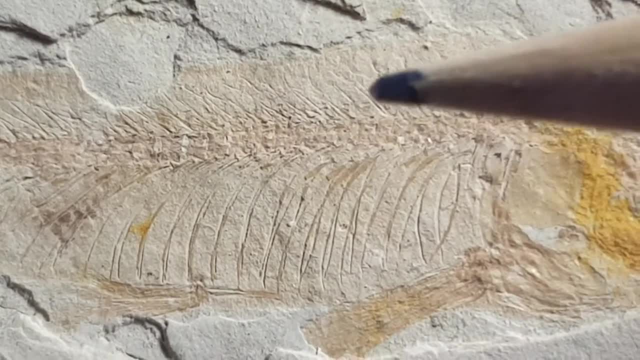 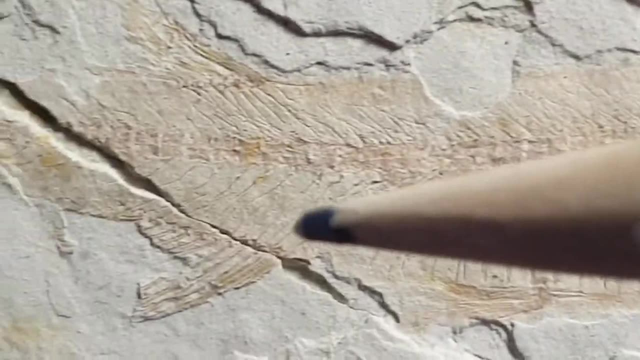 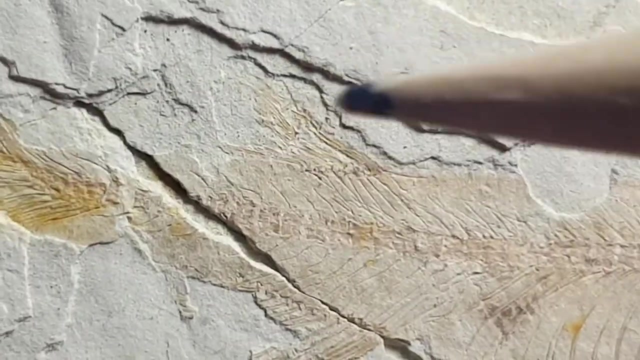 And the abdominal vertebrae is pretty much part of the pleural ribs, So not as advanced as current fish. And, as you can see, I have no first dorsal fin, I just have the last one. So these only have one fin. 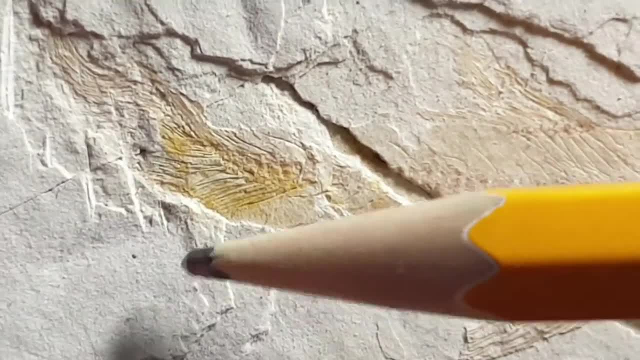 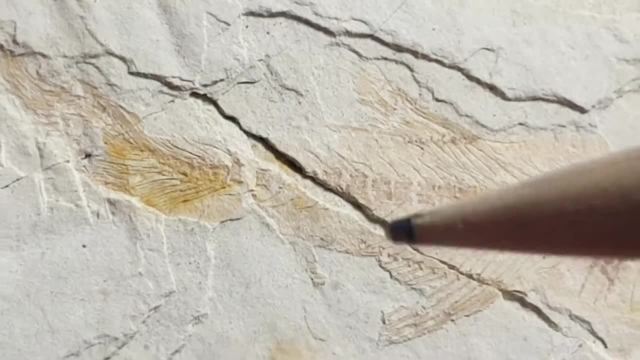 And then we have matrix here. So if I wanted to remove that matrix to reveal the actual tail, It will be good, But I'm not going to do that Because I'll probably damage it And underneath here it looks like there might be another fossil. 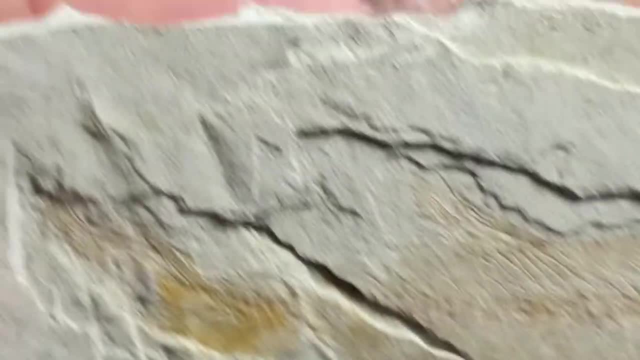 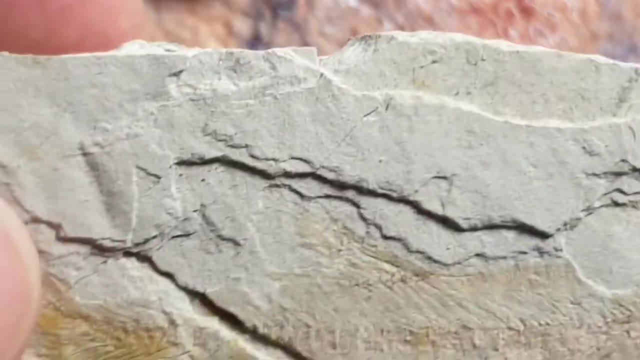 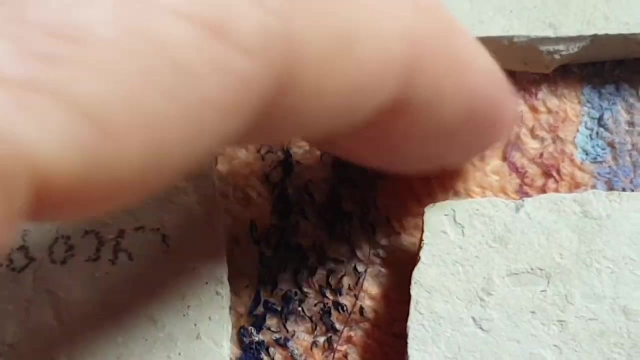 So this one looks like it's been broken in Put back together, Or maybe not put back together, But it's just been broken Because there's a lack of Removal of the matrix here. So that's a nice one, And the last one I've got is pretty much broken in half. 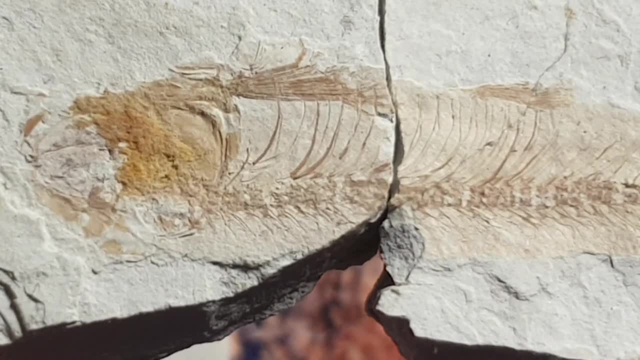 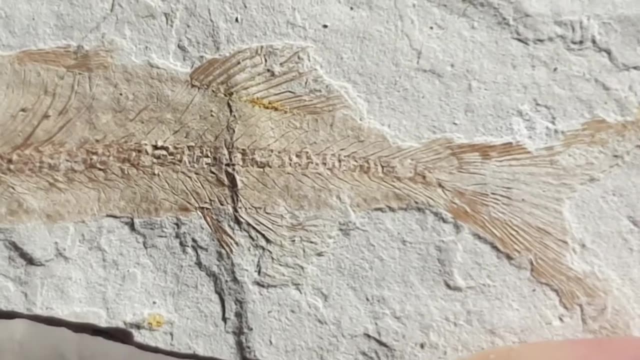 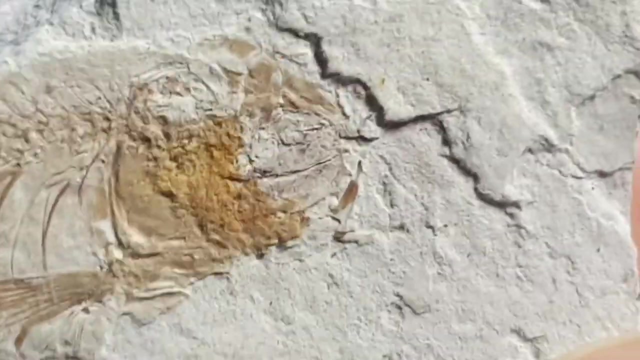 But it's a nice specimen. Got the top part. This is the top part, Then the bottom, which is broken, And we have the tail. So if you look at the head- Because the head contains so many bones They are Pretty hard to fossilise- 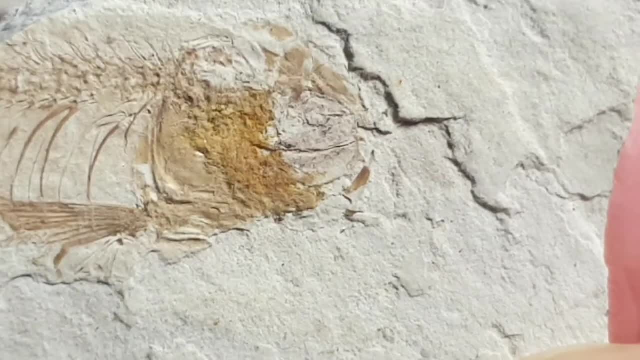 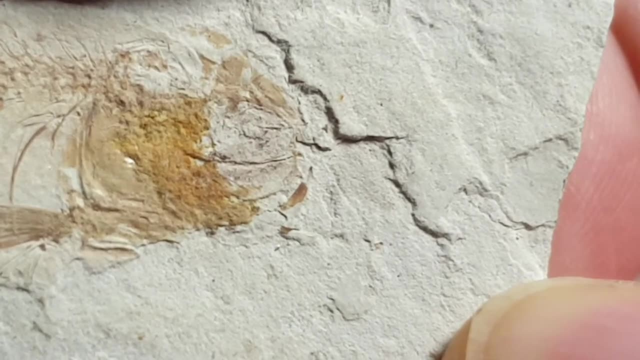 Because the head contains so many bones They are Pretty hard to fossilise Indistinct pieces. So You would need To put this under a microscope To actually reveal different types of bones, Because a lot of them are actually quite small. 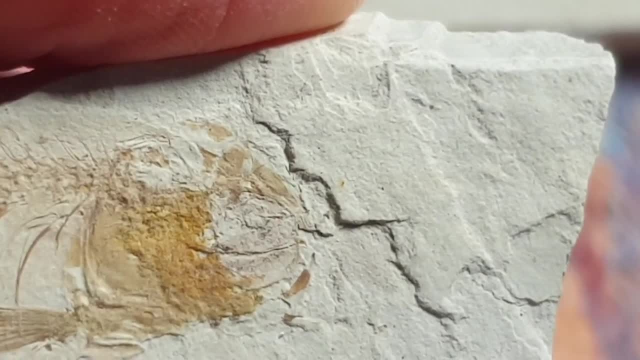 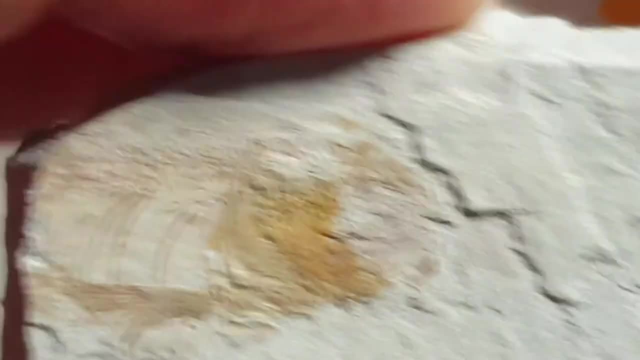 Because a lot of them are actually quite small. So you've got the parietal Should be up there. So the eye socket is in the front. It seemed to be quite large for this animal. It seemed to be quite large for this animal. 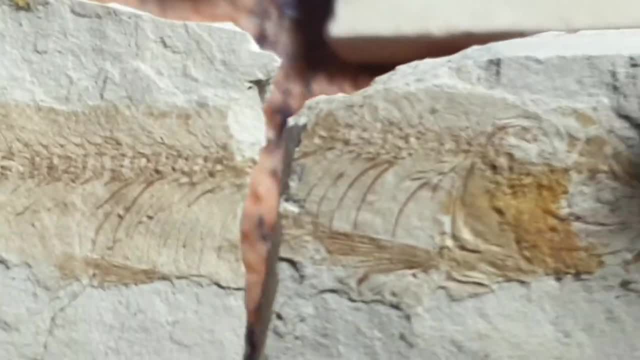 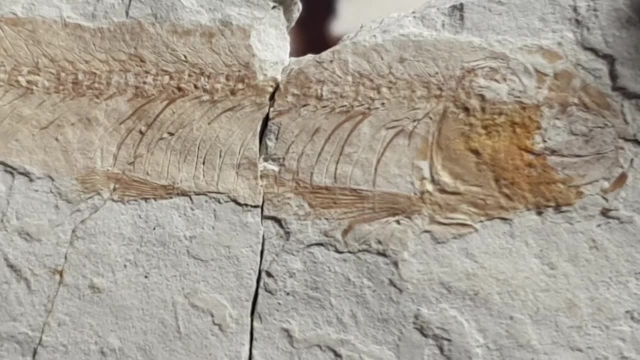 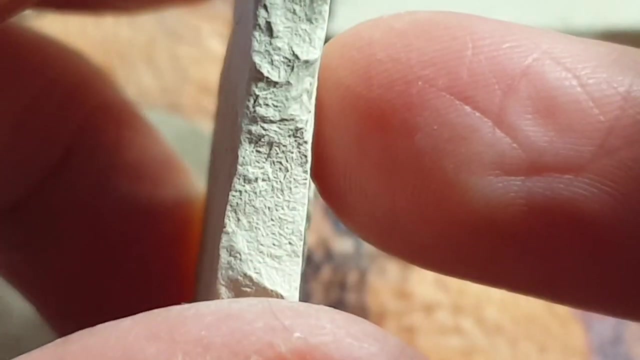 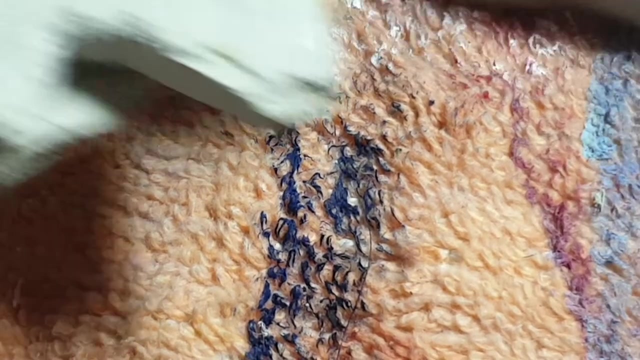 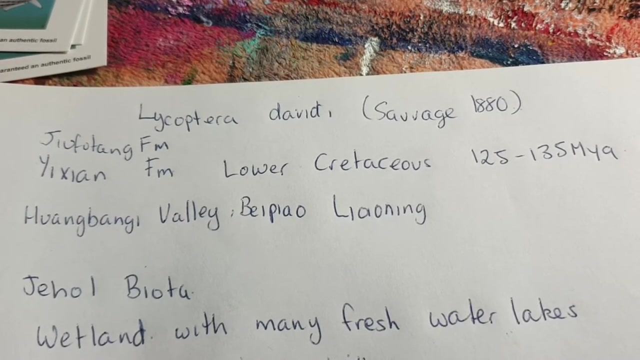 And this animal is supposed to be Like a common minnow and if we put it back together that's pity, so something like that. but if you look at the matrix, I don't think there's any other fossils in this slab, so these fish were okay. so here we have some basic information about these fossil. 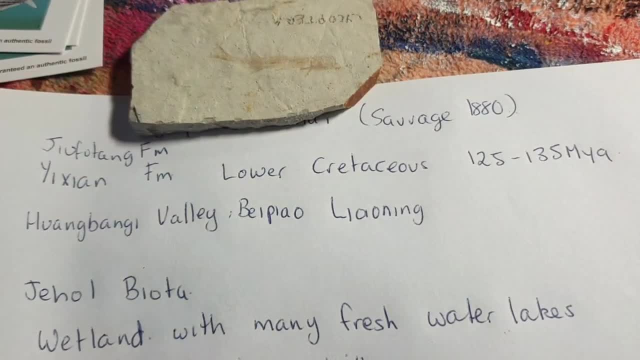 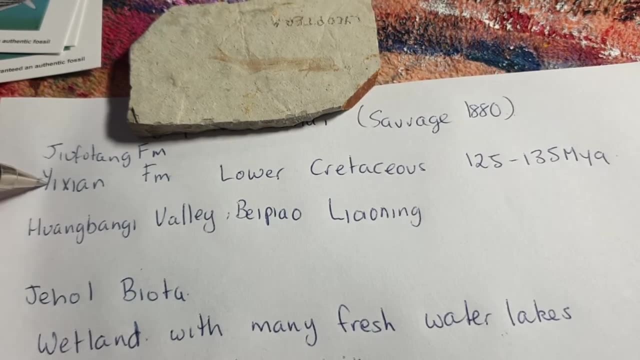 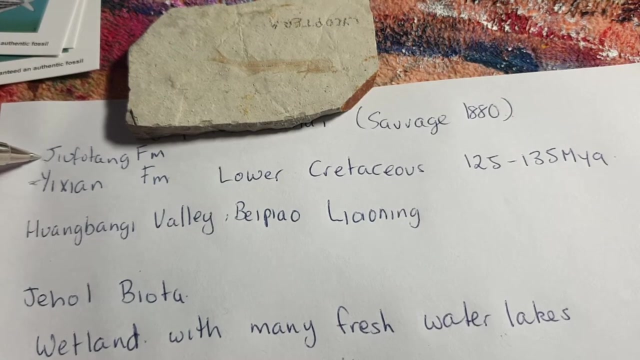 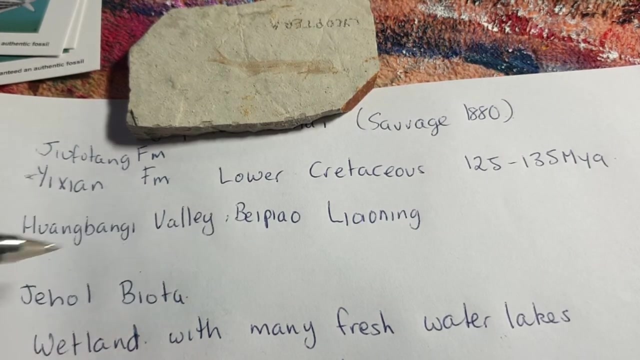 fish. so we have the formation. so this is most likely the formation species come in. this is the earlier formation in layer last. the later formation is the Yu Fatang formation, lower Cretaceous. it's in Huangbangi Valley in Baipao, China. it is a. 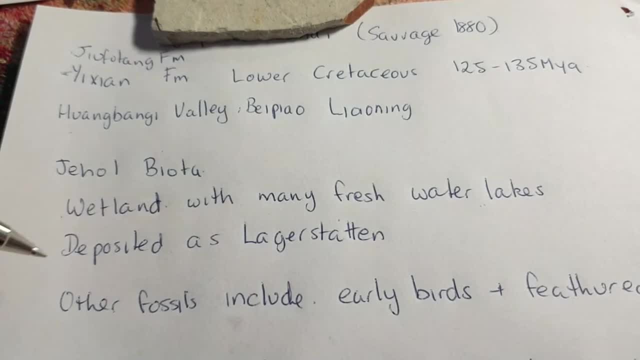 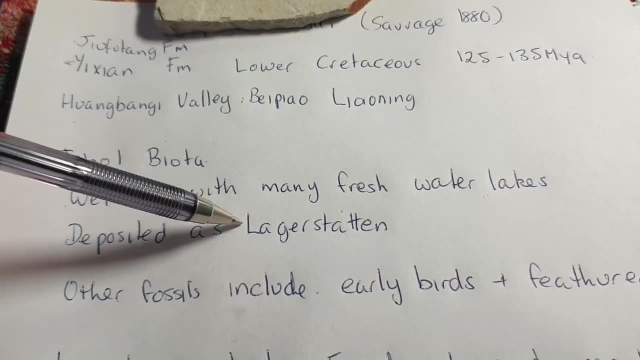 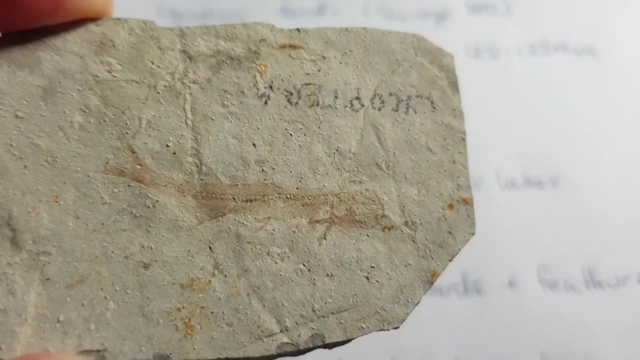 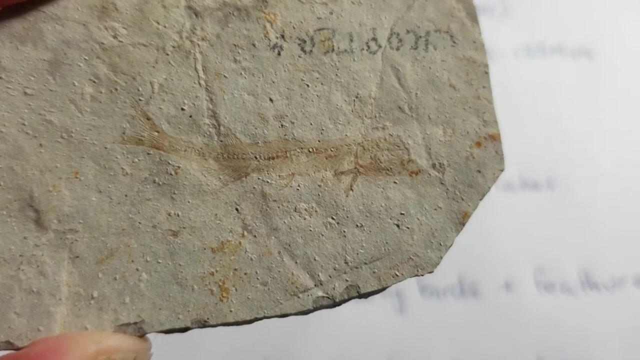 wetland with many fresh lakes, so it's probably shallow lakes. that's a Lagastatin, so that means the fossils are preserved quite well and these are found also with fossils of a lot of birds, pterosaurs, dinosaurs, other types of species of fish, a lot of insects. and also plants of fish, of fish and also plants of fish on the land. yes, this is my favorite one, My favorite, Moonática, and this is going to be this one. this will just be my favorite one. Ok, now I'm gonna go back to the poster and have a quick look at these, and I'm going to go back to most of the seas to see. 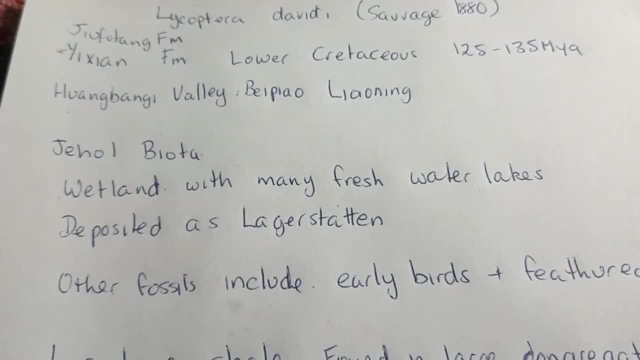 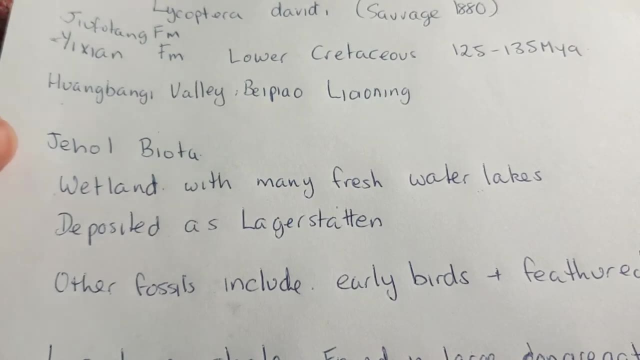 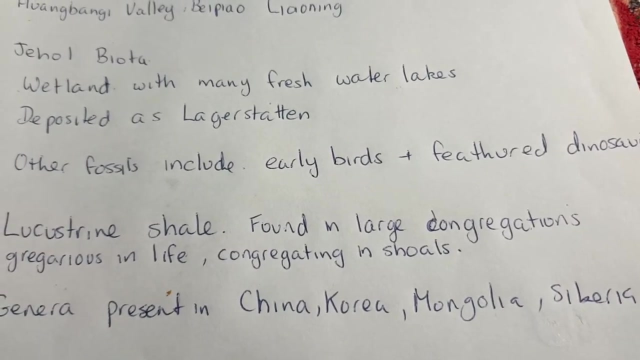 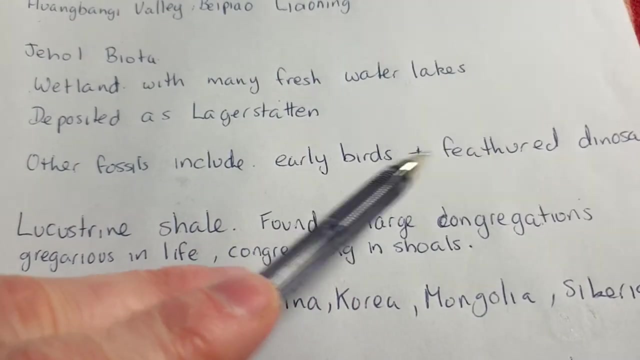 as well, so that's why it is a Lagerstätten. it contains a lot of other fossils that also can preserve a lot of other details, like internal organs, fine detail of the skin and other things like that. so you got feathered dinosaurs. so this is where we have made a very distinct connection between birds and 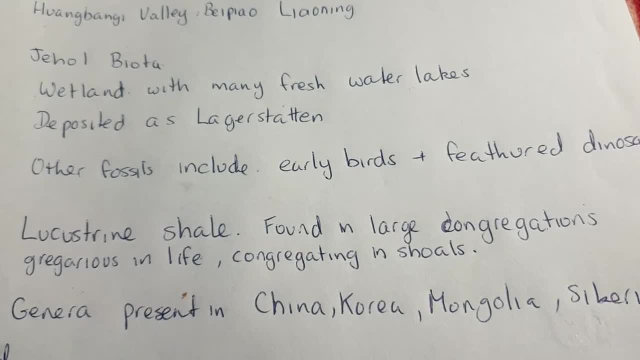 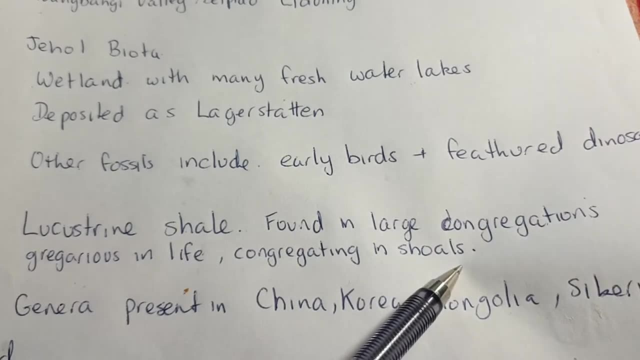 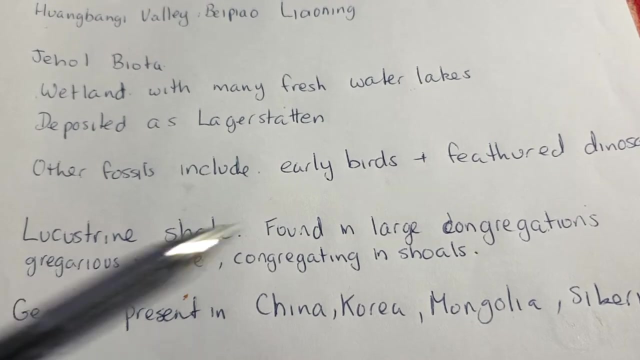 feathered dinosaurs is in these Chinese fossil locations. okay, it's a Leuchristein shale fending large cong, so the fish is fending large congregations. gregarious in life, so they're not solitary animals- and in shoals. so if you see a video, 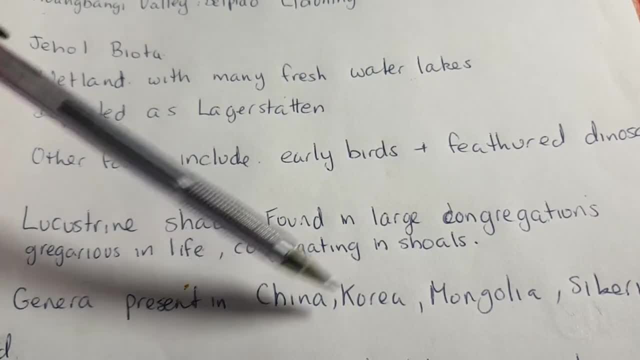 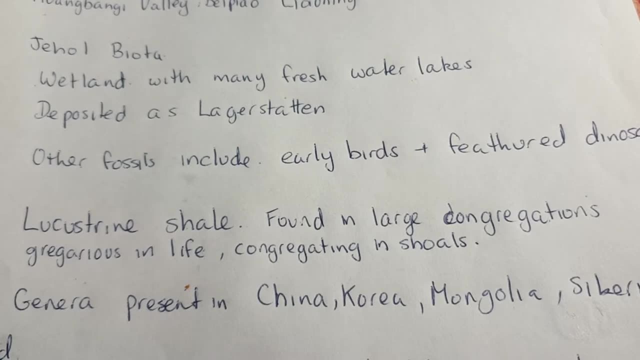 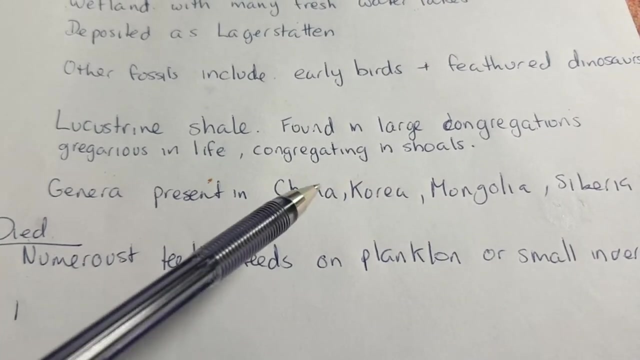 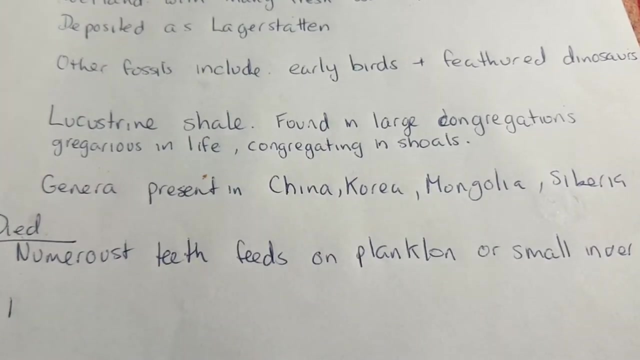 link in the description below where, like tuna, they like to swim together in large pools because there's a lot of predators and that would protect them from those predators for the most part. okay, and that's all this. genera Leuchristein is also fending Korea, Mongolia and Siberia, so it's pretty much over a lot of eastern China. 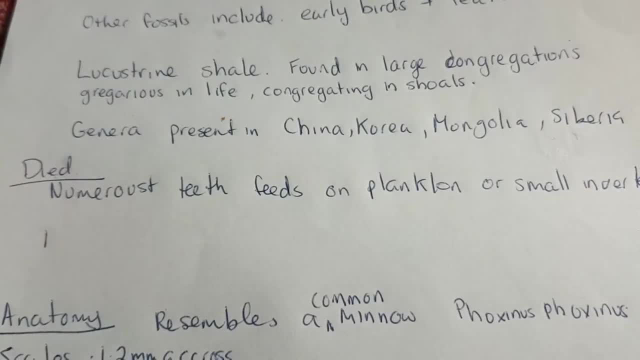 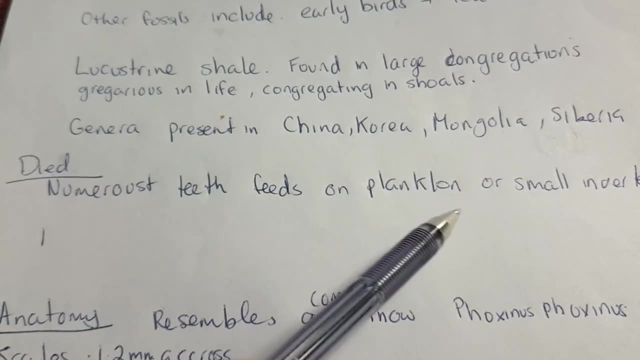 and yeah, that's it for this video and I'll see you in the next one. bye, bye. the only part of the anatomy I've found so far is numerous teeth, so I'm not too sure how many teeth they do have, and it feeds on plankton or small invertebrates. 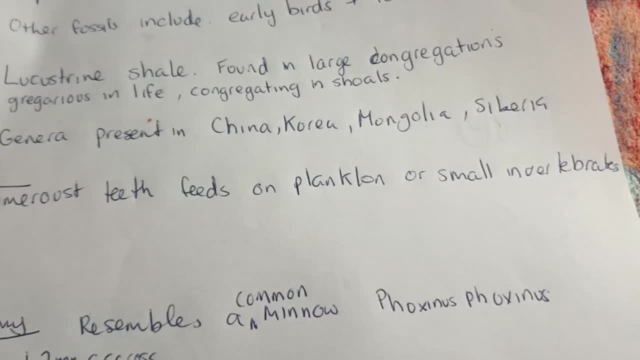 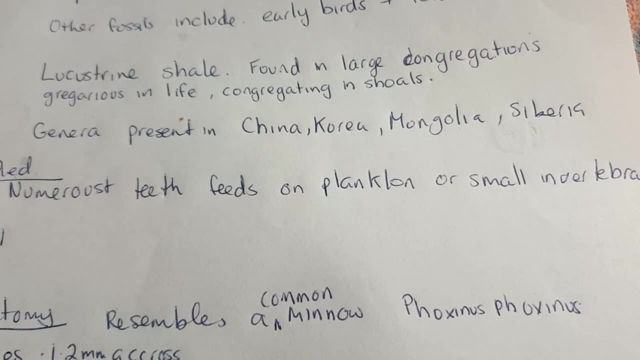 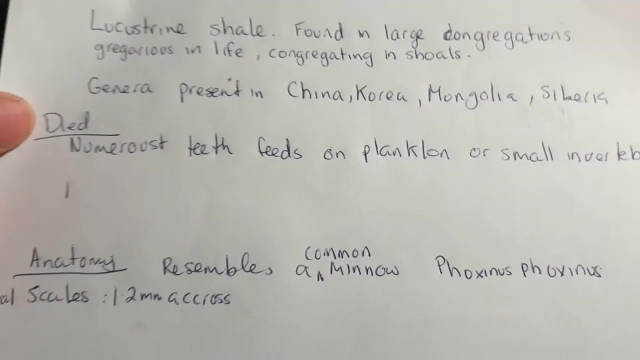 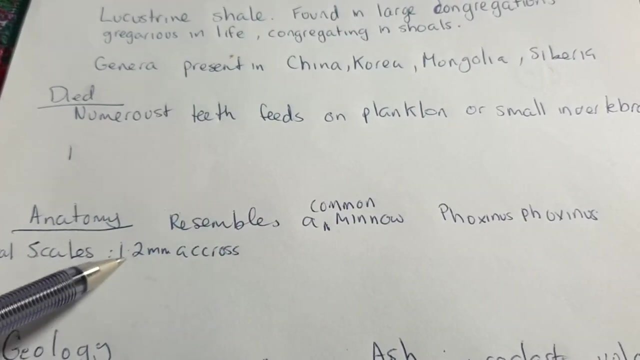 probably insects if it has small conical teeth. if it was to be shellfish, you would need to be. it need a lot stronger jaw and not pointy teeth. it's really not useful for shellfish. okay, resembles common, you know, and this is the species name. scales are usually 1.2. 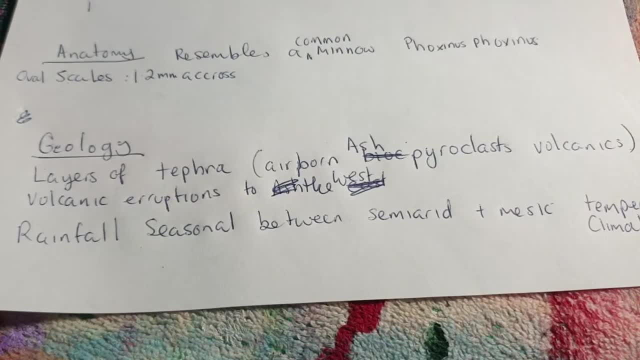 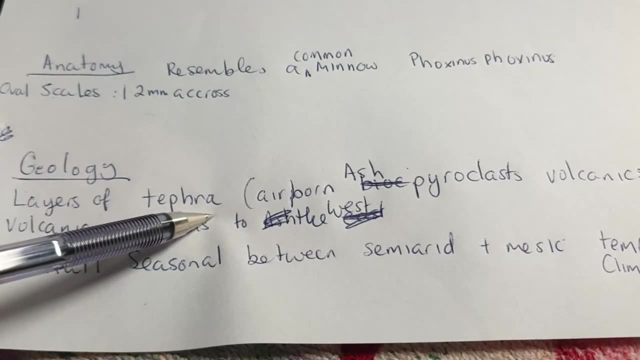 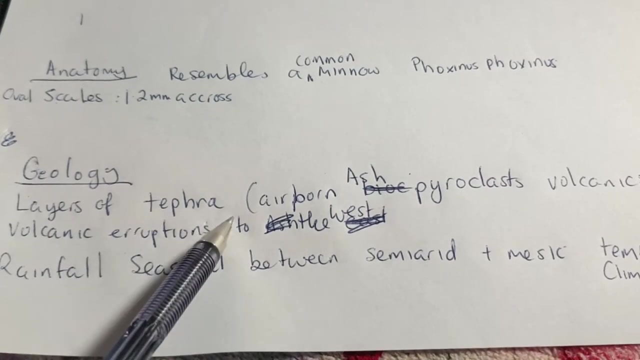 millimeters cross, so very small. okay, so we also have the geology. so there is a layer of tephra and also sandstone. so in between- and this is how they get, the age is from the tephra sort of volcanic ash- pro class of all mechanics, you do get a. 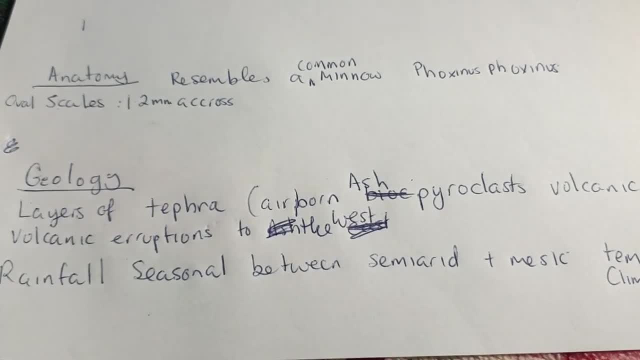 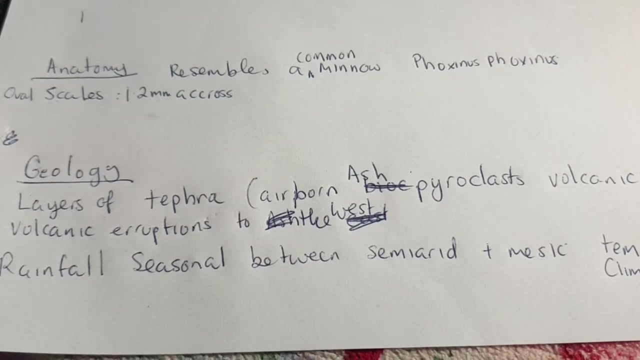 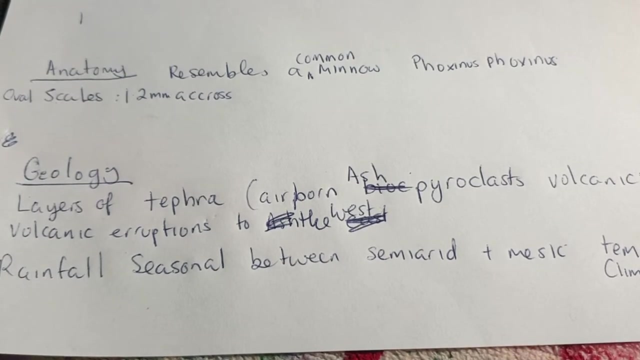 lot of volcanic bombs, larger rocks, but you know they probably wouldn't really occur and the volcanics apparently come from the West. I'm not too sure where in the West the volcanic seas, those volcanoes could probably have been a road by now. there might be some remnants of them, like. 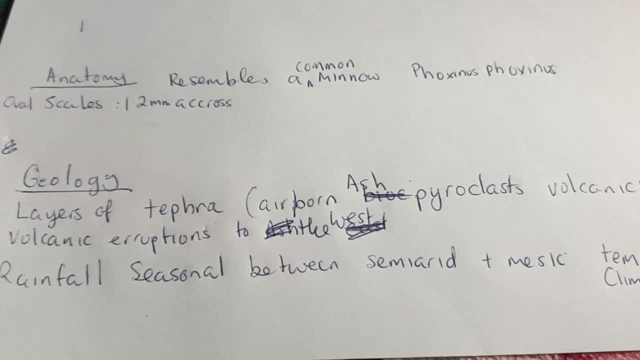 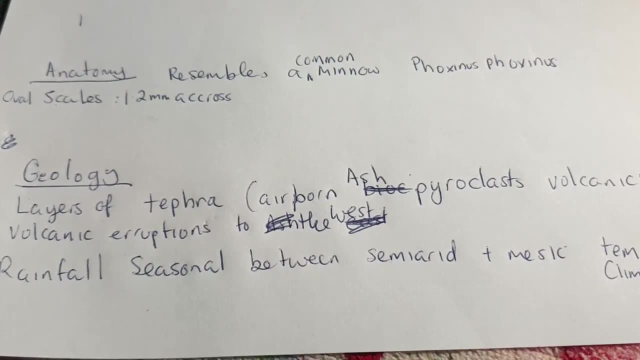 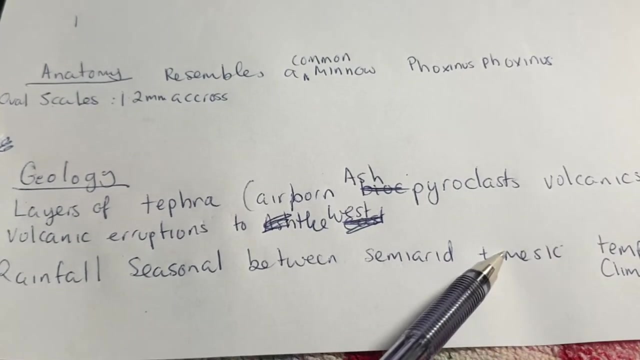 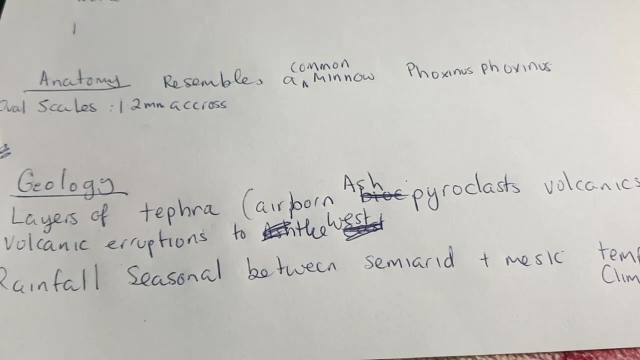 in we have. in Eastern Victoria. we do have remnants of volcanic flows from 300 million years ago and the rainfall was seasonal between semi-arid, so it's more likely in the summer, and mesic, so it's probably in the winter. temperate climate, so they do have seasons. in Melbourne we have a temperate climate in which we 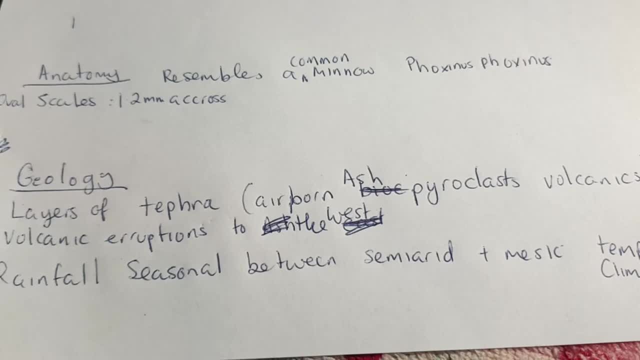 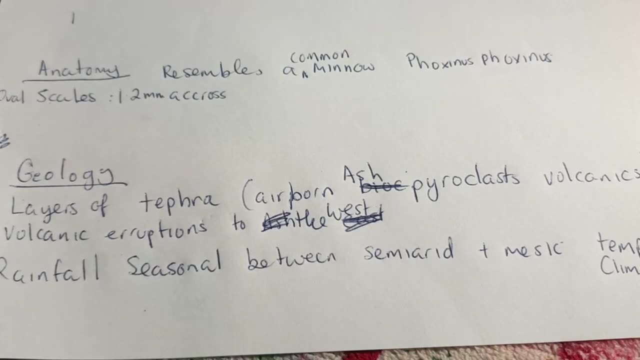 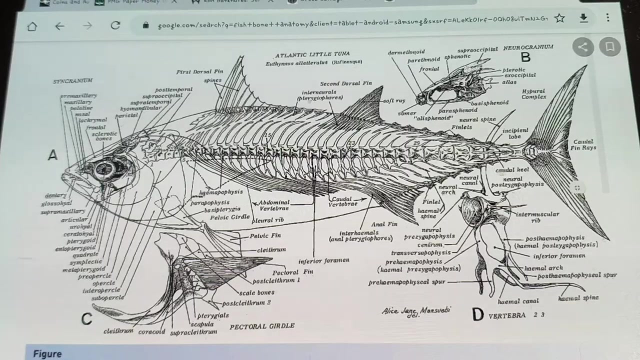 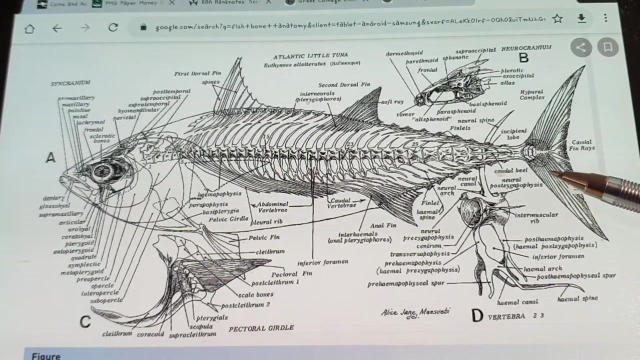 have a distinct summer and winter season, so that's more likely it's gonna be. and it rains a lot more in winter here than it does in summer. so that's the geological winner. just basic information of the actual species. so if you wanted to get the anatomy of a fish, here we have a tuna. it's more derived, so 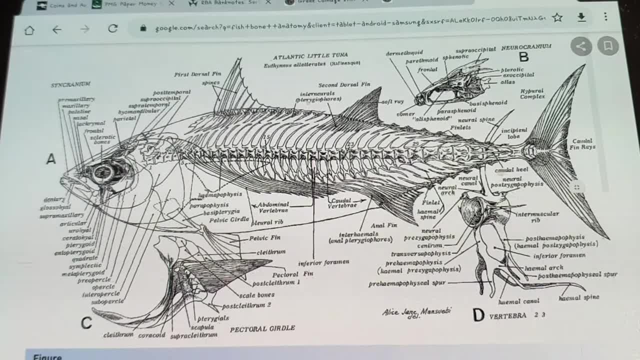 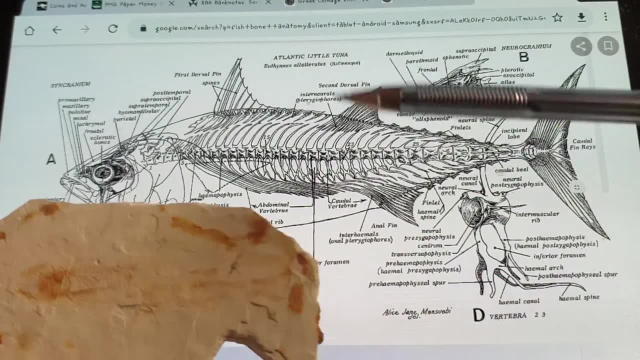 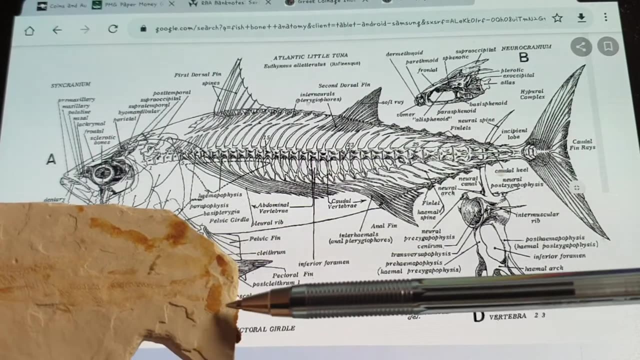 the. a lot of the anatomy that is present in these fossils will not be present in this fish. so we do have, we don't have, the dorsal fin, the first one, we have the second one and if you look at the vertebrae, vertebrae should be pretty much the same. 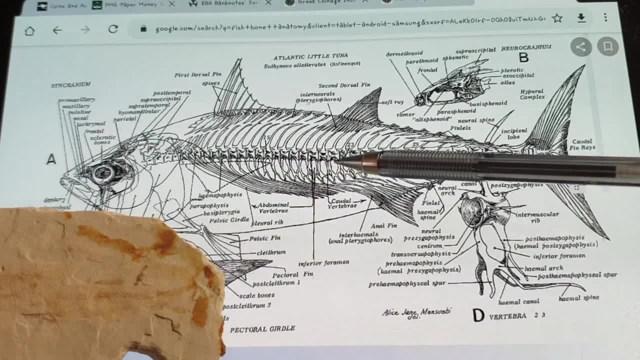 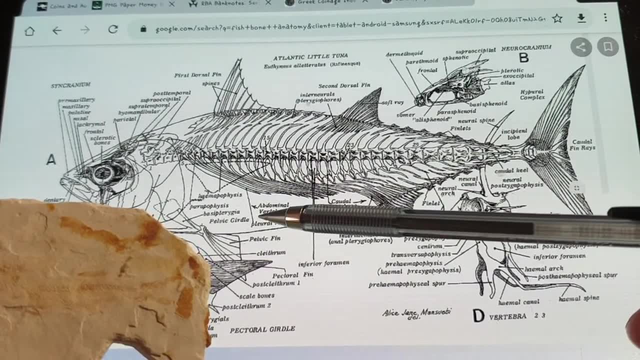 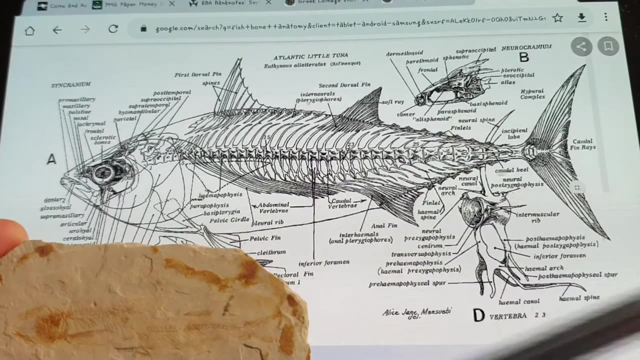 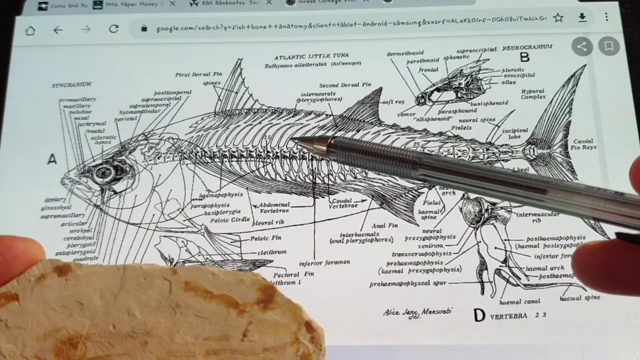 but we don't have this part here, so this is a like it. so here we have the abdominal vertebrae, the pleural ribs, and these vertebrae are more complicated then the vertebrae of this fish, and these vertebrae start up here. they're actually. 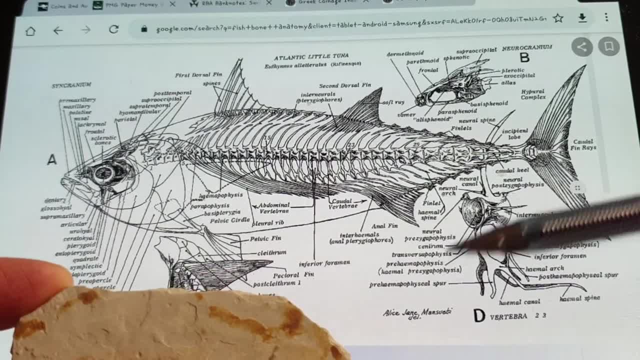 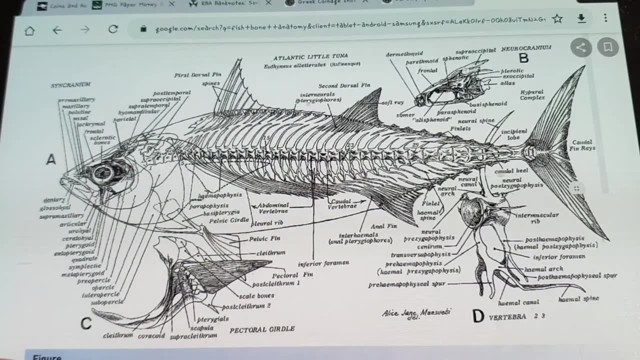 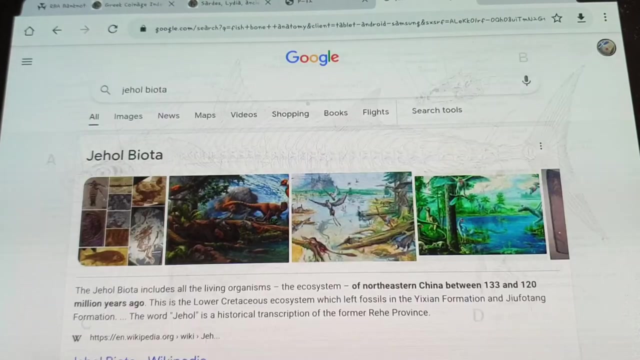 a lot smaller in this fish and then you got it looks like a more complicated tail. then we have here. but you know, this is just the basics. for every species you would have to learn a different type of neat and and if we go to information about this, so you get a lot of pictures here we 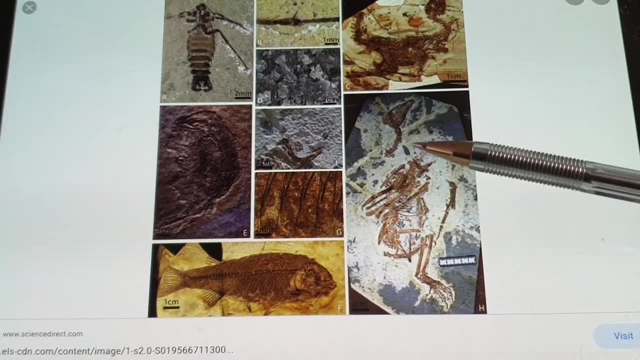 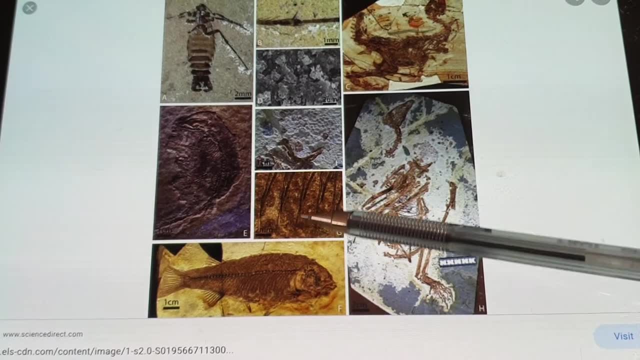 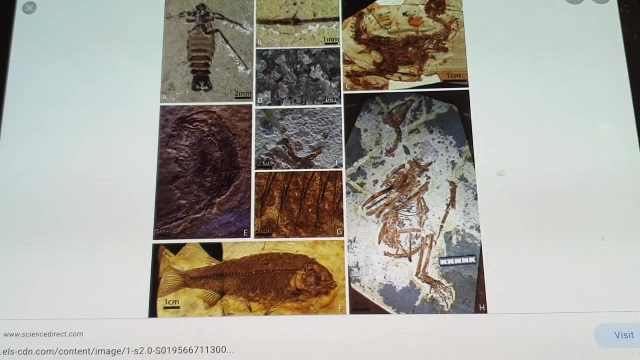 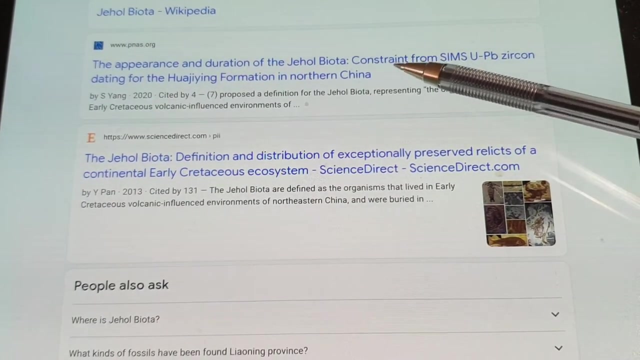 have. so we have a looks like a dinosaur, another dinosaur, fish, fish. this looks like a ribs. not too sure what those are: insects. that's probably the leg of the insect, but you get a lot of different information. but what you need to look at is the scientific papers. so we've got PNAS. this gives the age constraint. 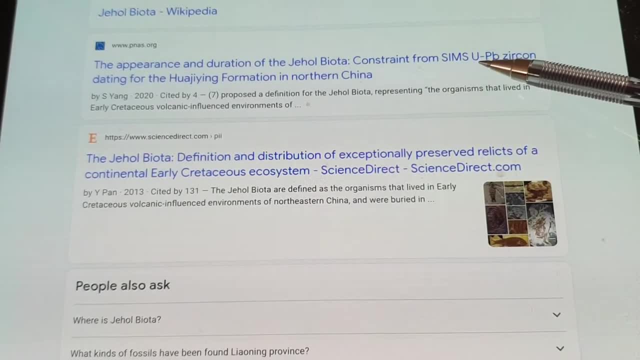 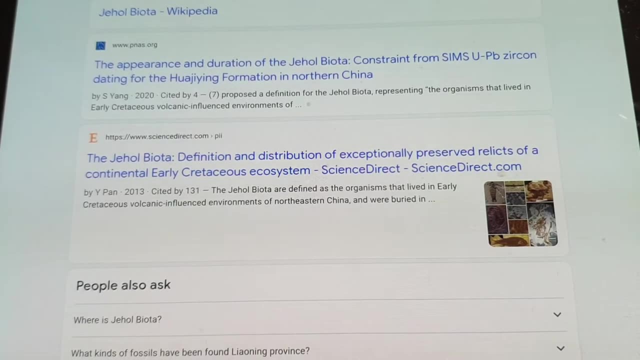 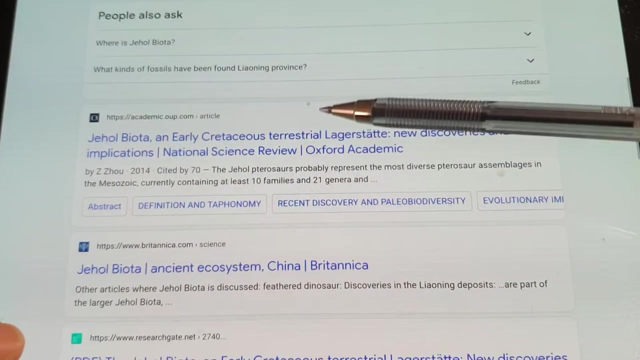 using uranium, lead. so uranium, because it's radioactive and it does lose neutrons and protons, it changes into another element in the last. last reduction in that series is lead. so it's a ratios between uranium and lead. and then we got, you know, distinction. then we got small G, whole biota. 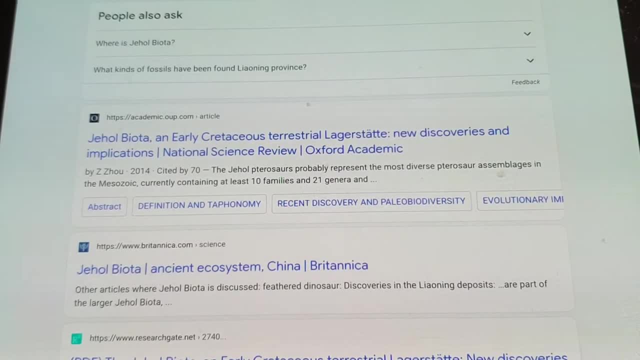 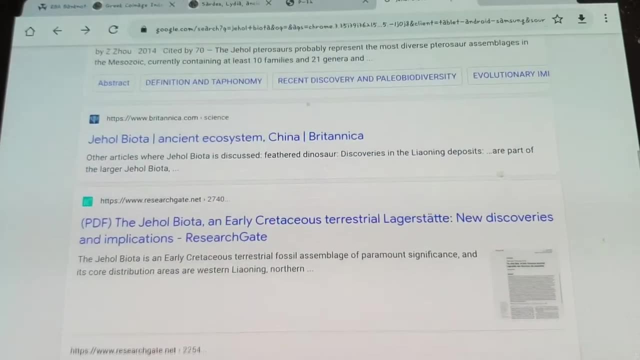 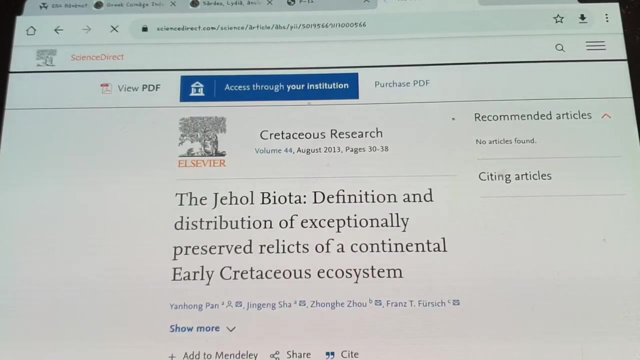 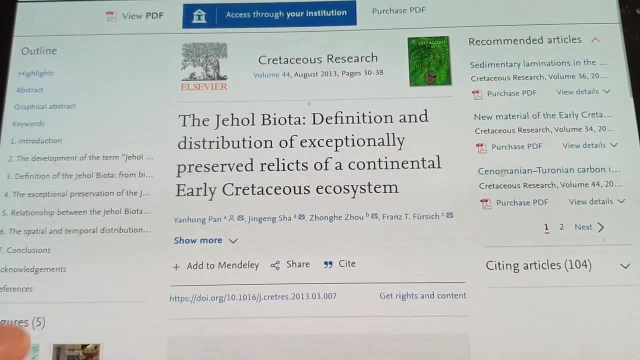 cretaceous, terrestrial like a city. so there's a lot of information that I'm gonna look at soon. so if you look at one science direct, a lot of these you need to purchase that's like thirty or forty dollars. okay, for nearly ninety years has been. 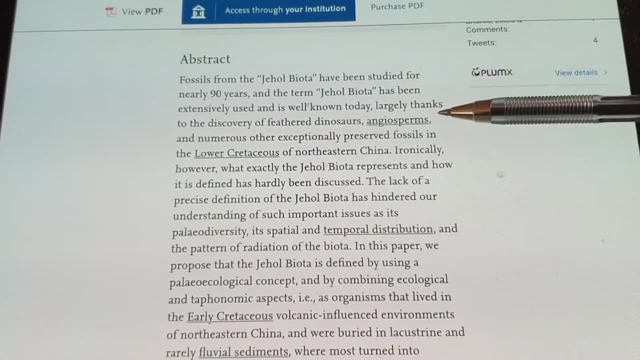 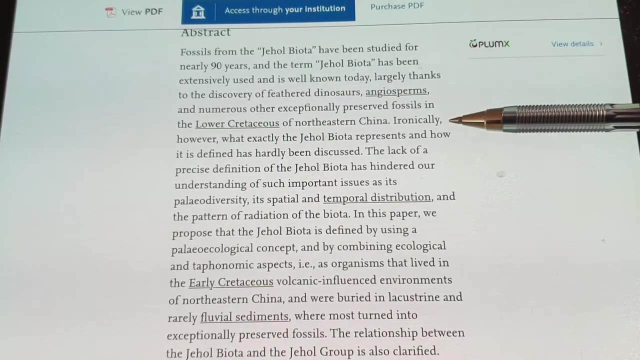 extensively used and is well known today, largely thanks to discovery of fever dinosaurs, angiosperms that are flowering plants. so the first flower and plants I believe come from this location, numerous, ever exceptionally grow, preserved for, from the lower cretaceous and overseas. then China, ironically have a ever what. 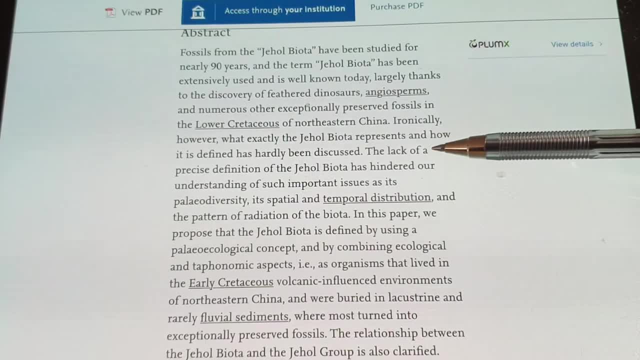 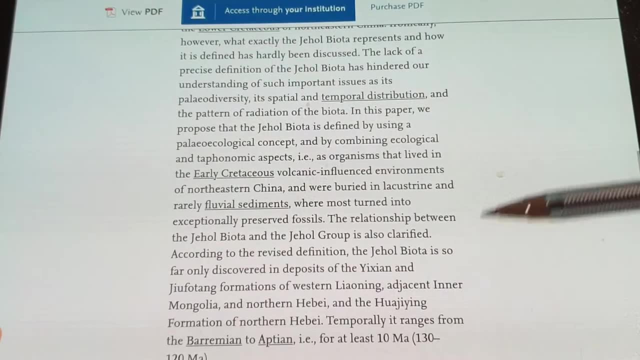 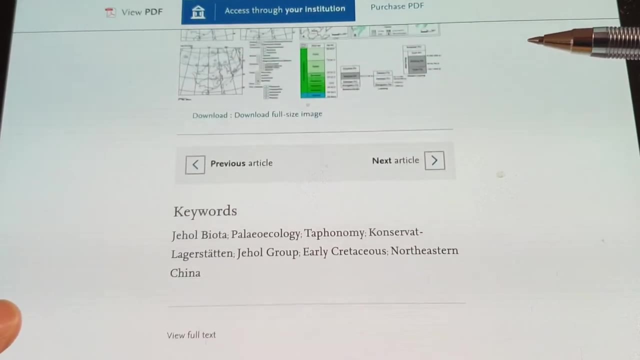 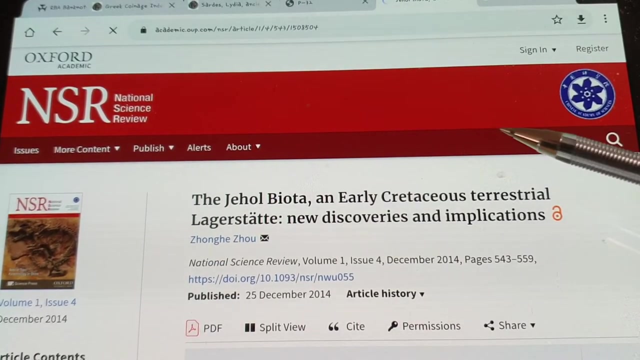 exactly the G whole bar to represents and how it is defined has hardly been discussed. okay, so they're trying to put a definition of this biota and they got lots of information, but you know you need to pay for it. then we have this paper. now you can actually read for free, so you can download it you don't pay for. 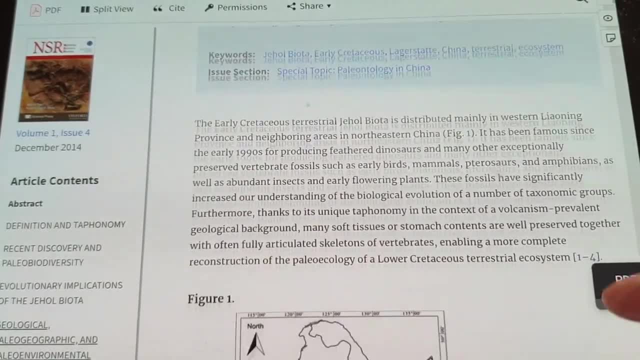 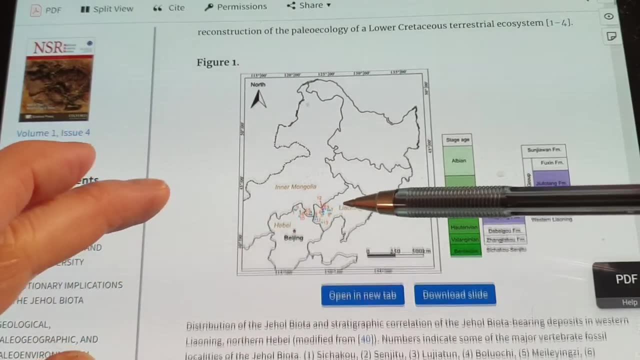 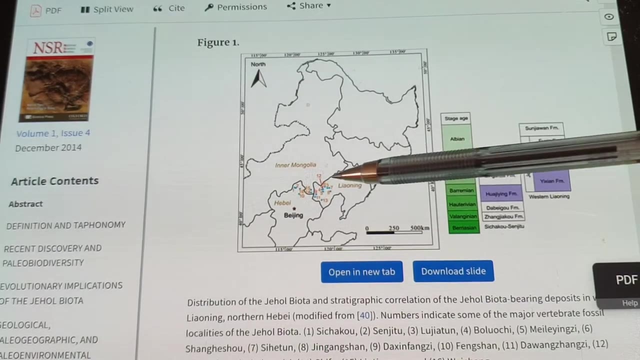 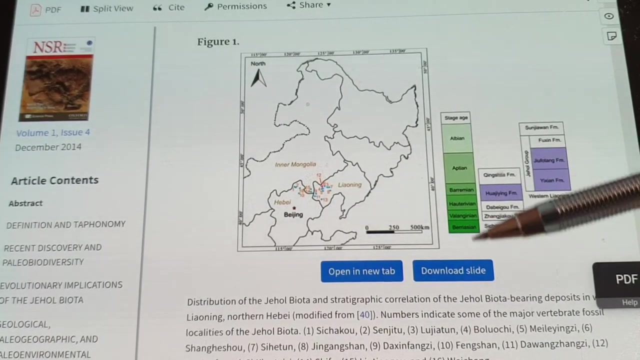 anything, but you can also just read about it in here. so here we have the fossil site. so there's quite a lot in his Beijing. the capital, North Korea is here, so this fossil formation is more likely. it's supposed to be in North Korea as well and if we go down, there's a lot more information if you want to read. 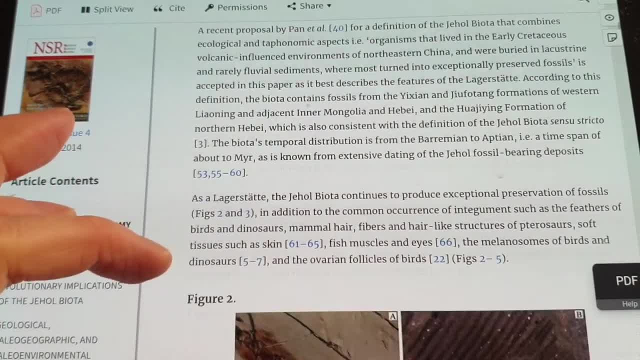 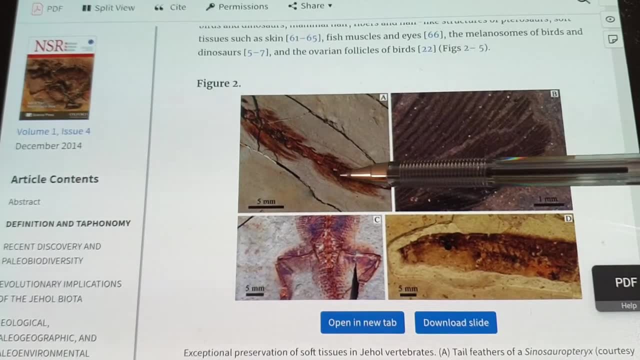 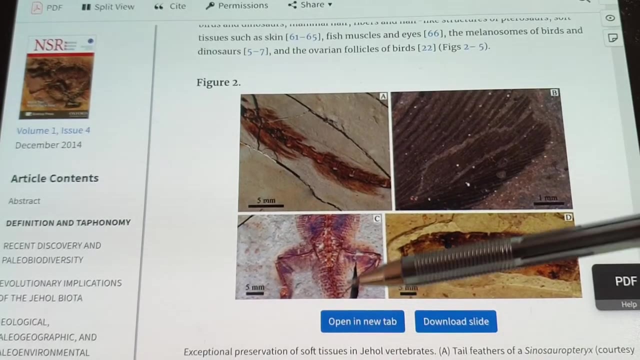 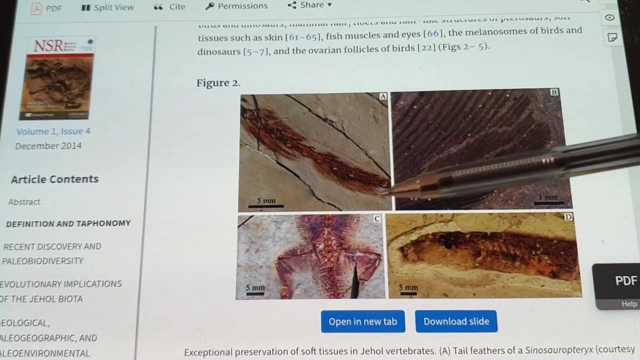 this paper and just look up G whole, whatever. so then we have some. so we got a tail feather on synopsis or Terex, so a bird or a dinosaur. so we got a tail feather on synopsis or Terex, so a bird or a dinosaur. flight feathers of Confucius soanus, so that's that one skin of a lizard, Neil. 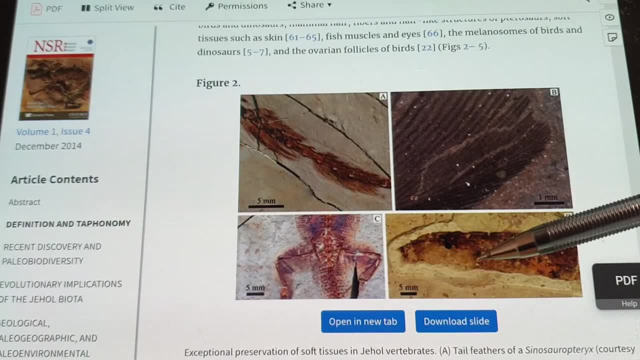 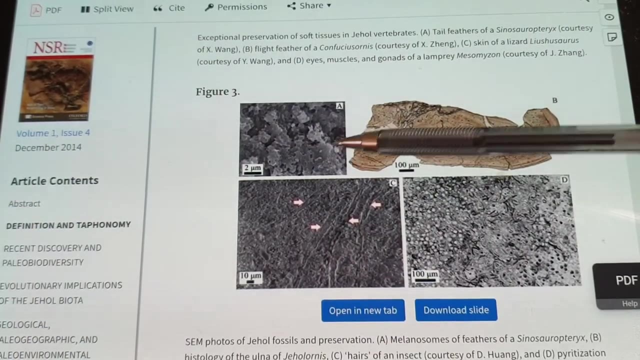 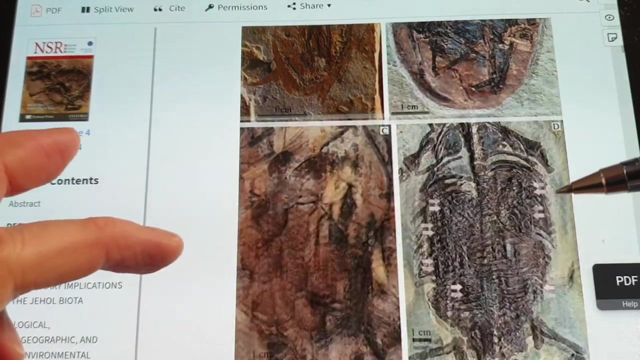 shoesaurus and the eyes of a lamprey, itself primitive fish, meso mizzen. nah, lampreys are not fresh, the lampreys. and here we have some more fossils. it's quite interesting. this one definitely is a good read. and here we have a pterodactyl. 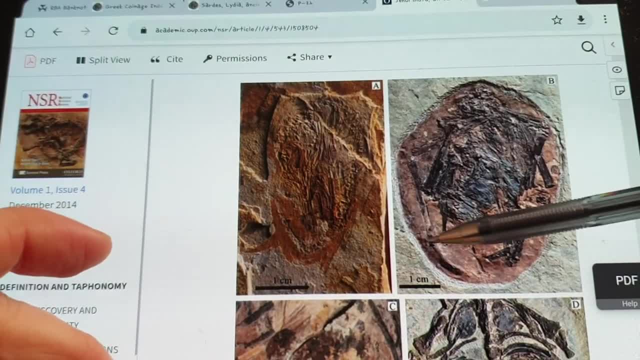 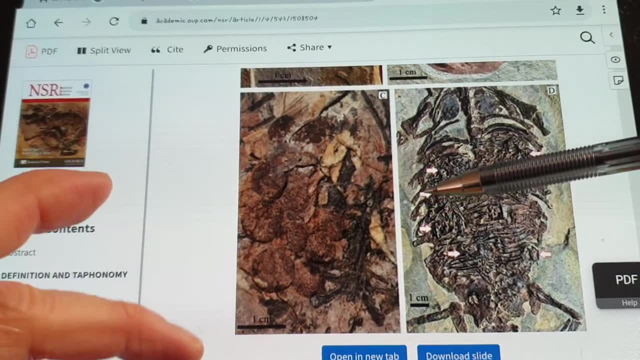 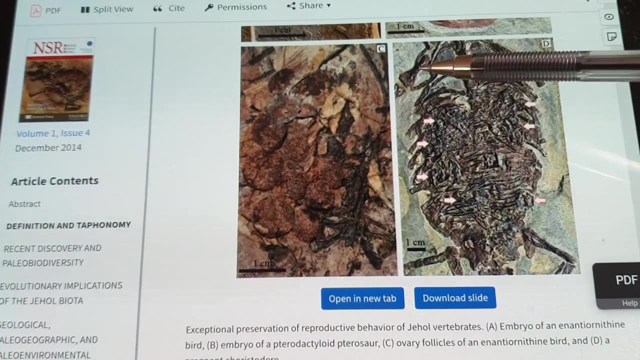 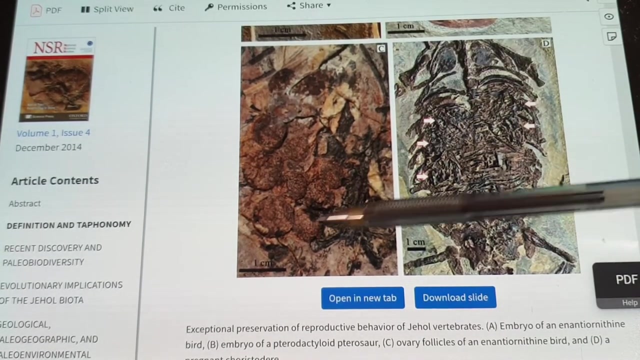 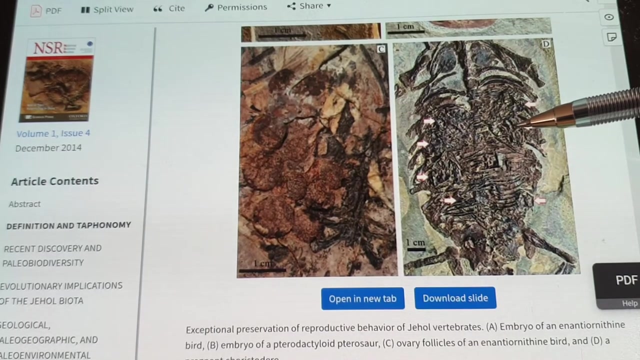 pterosaur, so that's B, so it's an embryo and egg. what's the first one is another embryo of a bird, so that's a bird pterosaur. they both laid eggs and then we have every follicle of a another bird and a pregnant bird. I believe that's a.